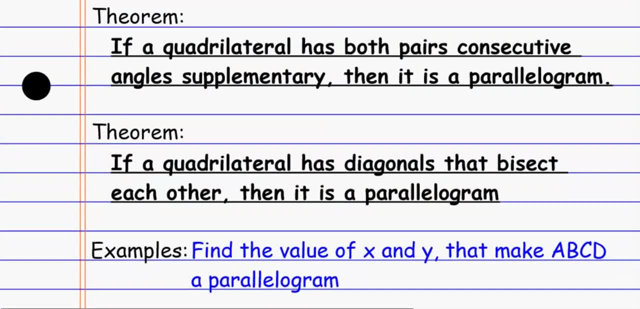 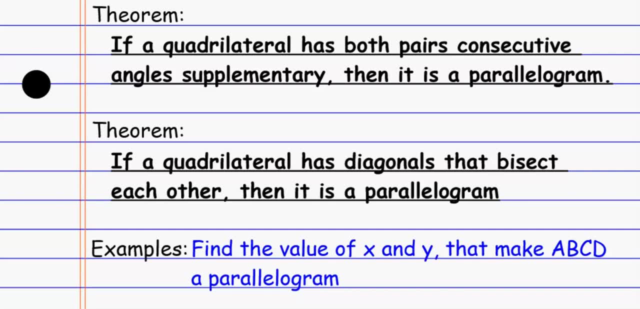 go subliminary. I can go backward and say it's a parallelogram, okay, And then the other property we have is that the diagonals of a parallelogram bisect each other. So if I have the opposite, if I have diagonals and a quadrilateral that bisect each other, I can go backwards and say 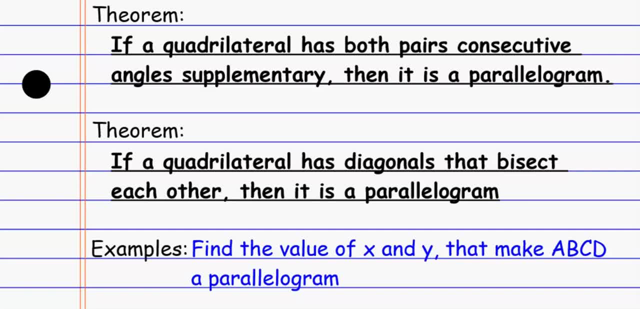 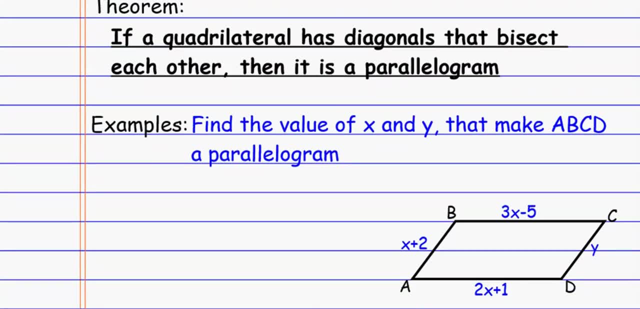 the thing is a parallelogram, So it's all those same properties, We're just using them in reverse, okay. And so kind of think about it from that perspective. If I looked at something like this, find the value of x and y that make a, b, c, d, a parallelogram, okay, And so I don't know if this 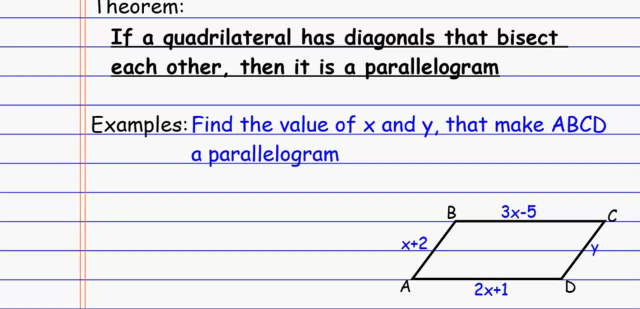 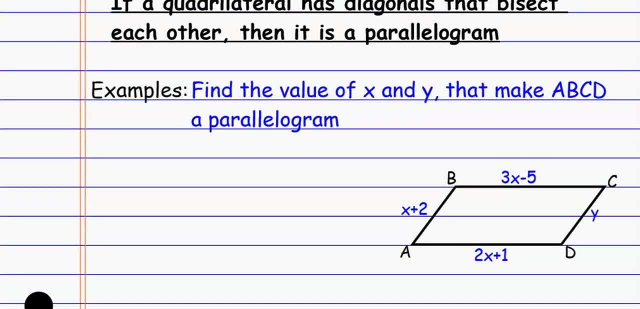 is a parallelogram. but what values would make it a parallelogram? Well, if I were looking at this thing, if opposite sides are congruent, it would make the thing a parallelogram. So, if you know, y were to equal the x plus 2, and if the 2x plus 1 were to equal the 3x minus 5,. 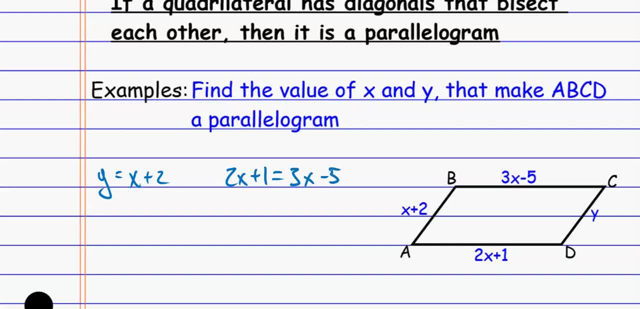 then that would make this thing a parallelogram, because it would make the opposite sides congruent. okay, So it's the same questions we've been answering, but just from a different perspective. okay, And once again, this guy, as I kind of went through this, you could look at this: 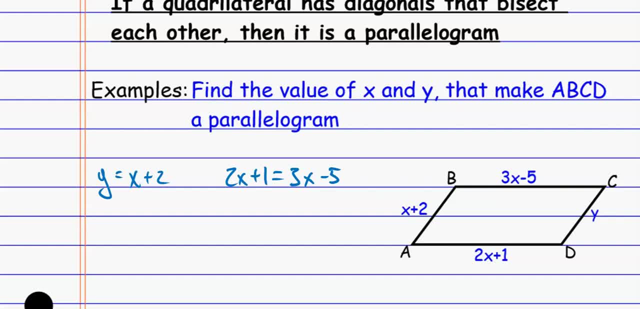 almost like a system of equations. but look at that second equation. It's all x values. And so here, if I subtracted the 2x from each side and then added that 5, gives me a 6.. Now I have to. 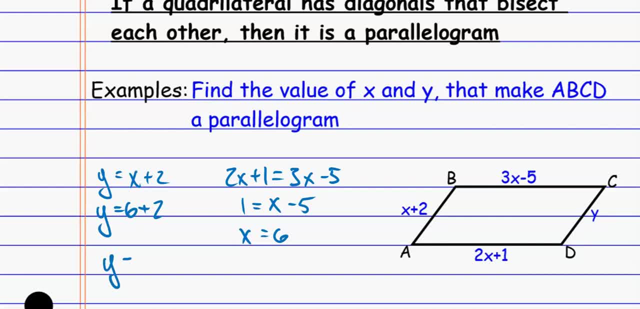 plug it back in over here. Okay, that's it. okay. So we're just looking at it from a different perspective. Before we were saying, hey, this is a parallelogram, so these are congruent. Now we're saying: 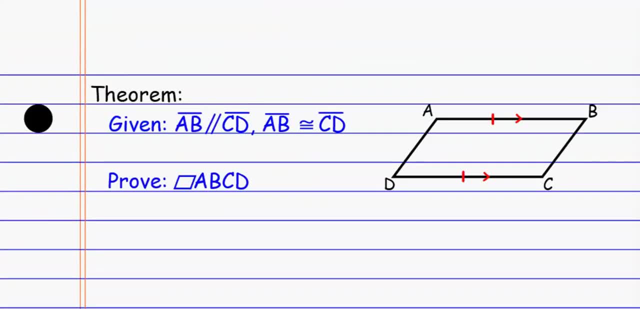 if these are congruent, then it would make it a parallelogram. All right. so here we're going to have one special theorem for proving that quadrilaterals are parallelograms. that isn't directly one of our properties in reverse, So it's not a converse of one of our properties. 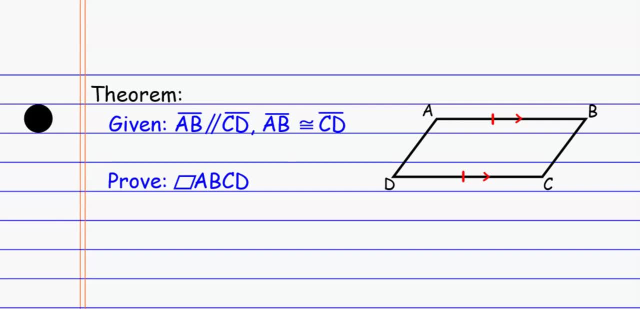 So here I have that I have one pair of opposite sides parallel, So I have AB is parallel to DC or CD and I have that that same pair of sides is congruent. okay, And this is a little bit different We're used to. 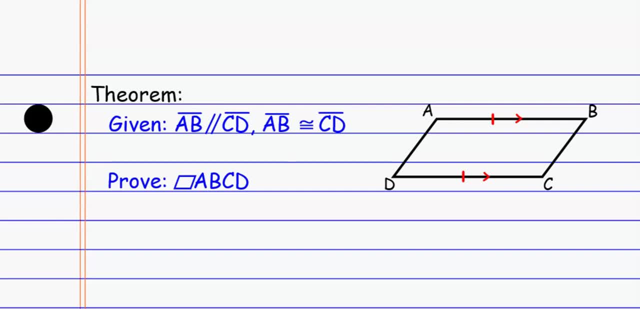 having two pairs of opposite sides congruent. Now, I only have one pair, but I have, in addition to that pair of opposite sides being congruent, that those opposite sides are also parallel. okay, And so, with just that information, I want to prove that this thing is a parallelogram. So this is. 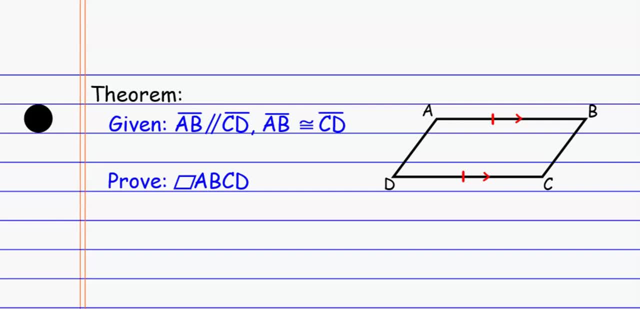 kind of a special one That's not quite as obvious as the others. The others are really obvious because it's just the reverse of our properties, This one's kind of special. And so as I kind of start to think about this proof and start to map it out, really I don't have a lot of information as I look at this. 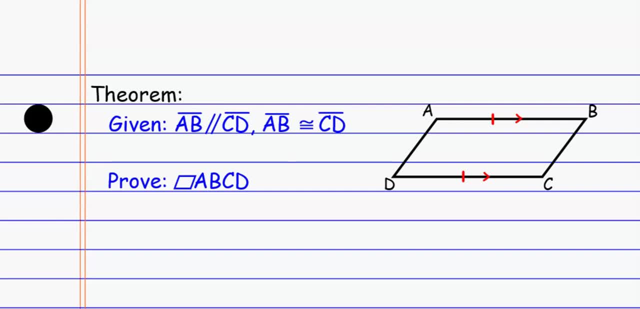 thing from the perspective of just having parallel sides here and congruent sides. So I'm going to have to draw an extra piece, as I have to sometimes. So I'm going to draw a diagonal. Wow, I completely missed. Let me try again. I can do better. I believe in me. Let's go red. That was the 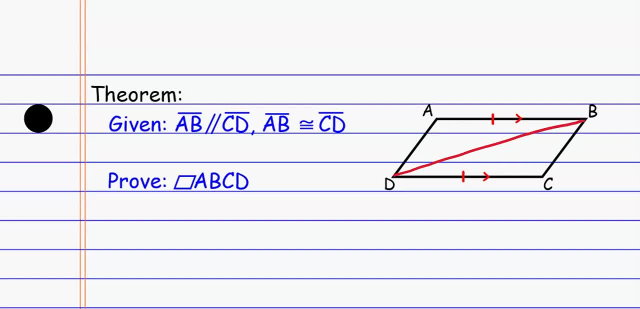 problem. I tried drawing in blue, Silly, Mr Jansen. But anyway, if I look at something like this guy now, think about this from the perspective of looking at the two triangles, and we should be able to come up with this thing being a parallelogram. okay, And so as I look at something, 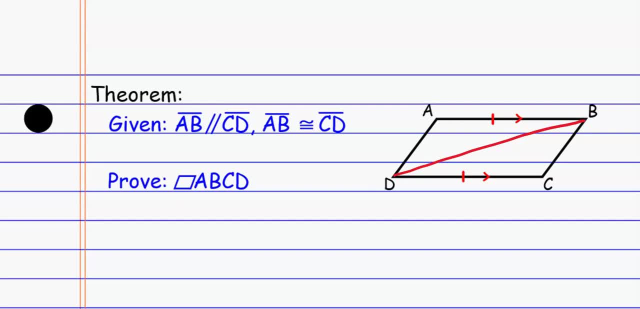 like this guy. the first thing I would probably do is I'd probably label some of these angles like this one and this one. okay, I'm going to call that angle one and angle two. And so if I use those side pieces, AD and BC, if I just look at DB as a transversal connecting those two, 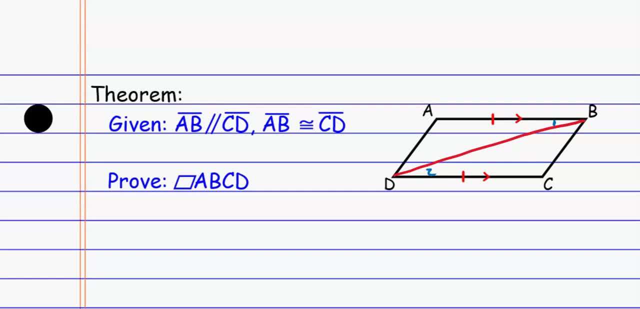 parallel lines. one and two are alternate interior angles And so if those are congruent and the sides I already have are congruent- and I know that DB is congruent to itself- I already have the three pieces I need for the triangle. So let's put this into a proof. So I've got my statements and my. 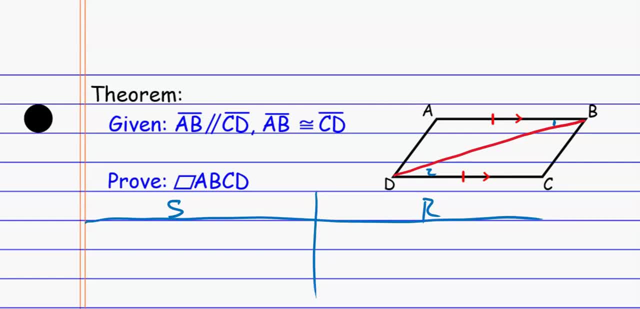 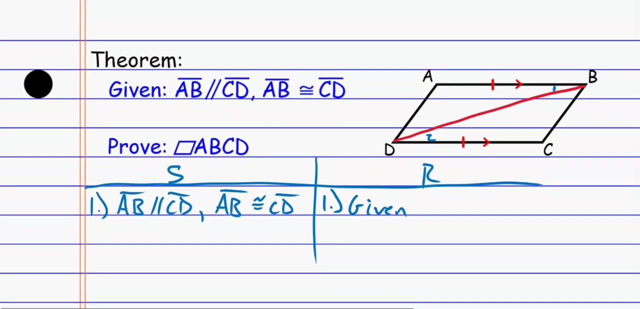 reasons here And again, that's given. So I'm just going to say that it's given. all right, I was given those pieces of information And then from here, and you know we could include that- hey, we drew a DB. 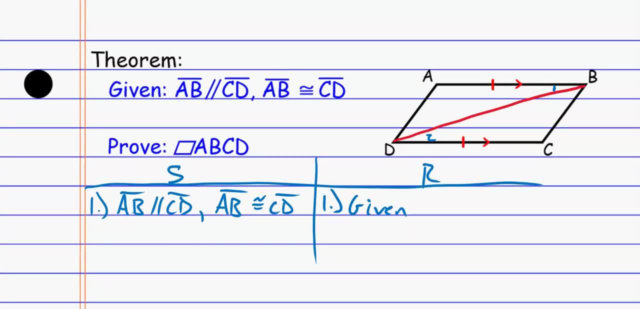 all right, I think it's okay that we kind of just showed it off to the side. If you want to put it in here as step two, I constructed diagonal DB, that would be okay. I'm going to go right to just saying: okay, well, if I draw that thing, 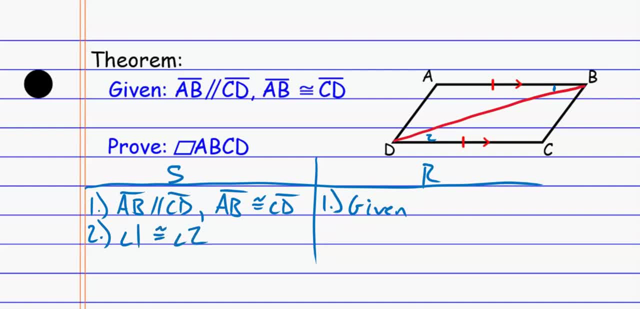 I know that angle one is congruent to angle two And that's because of alternate interior angles of parallel lines. Okay, so alternate interior angles of parallel lines are congruent, And then from here I could say that something like DB is congruent to itself, and that's my reflexive property. 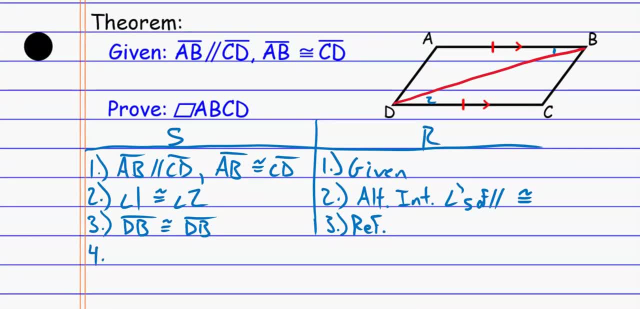 And so now what I have is: I have the two triangles are congruent. So from here I could say that triangle ABD is congruent to triangle. let's see C. I got to make sure I label it in the same fashion, DB. 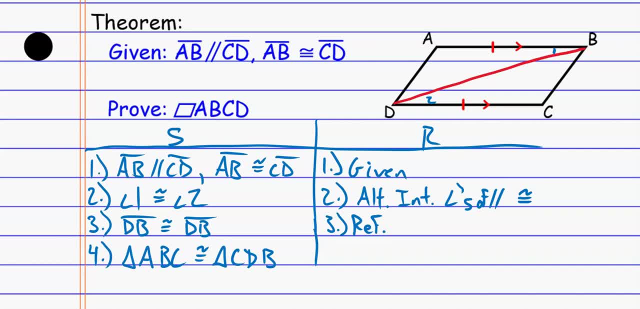 And those two triangles are congruent because of side angle, side As I look at this thing and maybe I can label it up here, those two dashes. So right here I had side AB, then angle one, then side BD. In the other triangle I had kind of the same thing: CD, angle two and then DB. 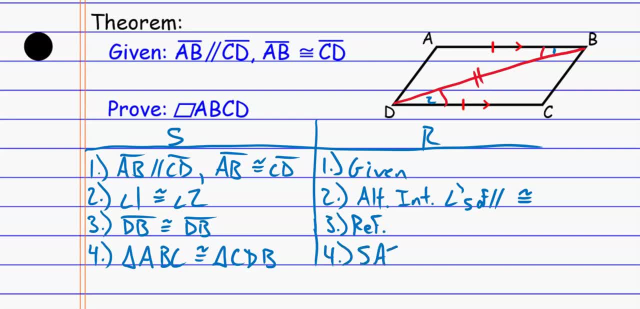 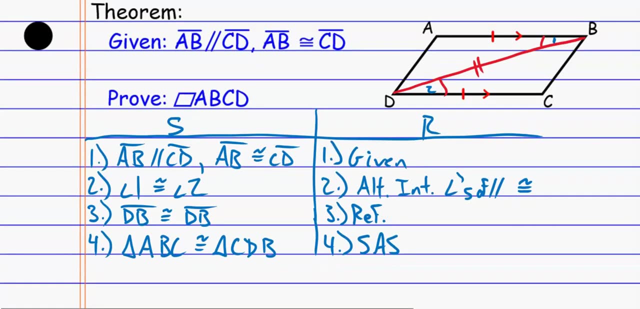 So side angle, side, And now, if I know those two triangles are congruent, I know all their pieces are congruent, And so there's a bunch of routes that I could go here, but the shortest one is just to go right to those opposite sides, AD and BC- and use that property. 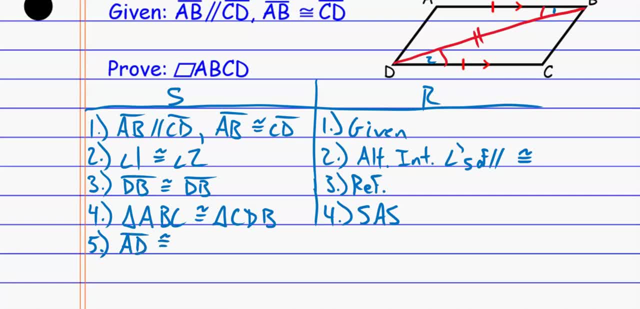 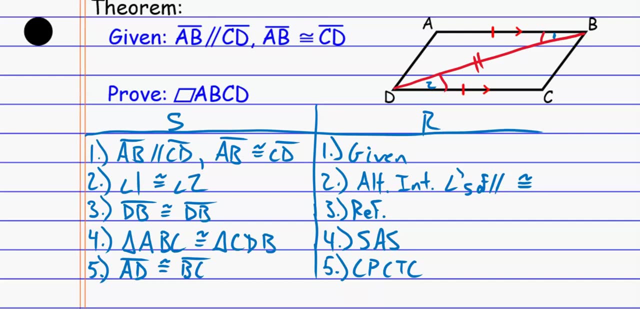 So I'm going to say that AD is congruent to BC and that's CPCTC. Okay, And now, if I have those sides congruent, now I have both pairs of opposite sides congruent, which allows me to say that this thing is a quadrilateral or, sorry, is a parallelogram. 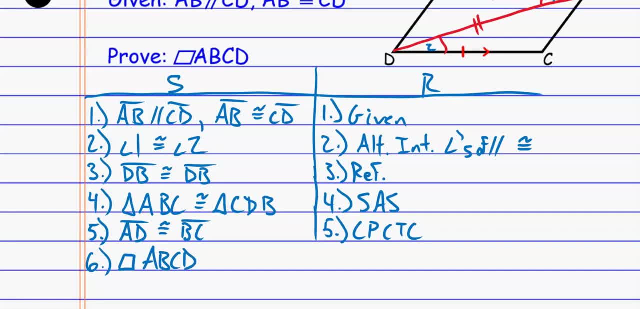 So now I can prove that ABCD is a parallelogram and that's because opposite sides congruent, so it's a parallelogram. Okay, And that goes back to one of our other values. So think about what that's done for us. 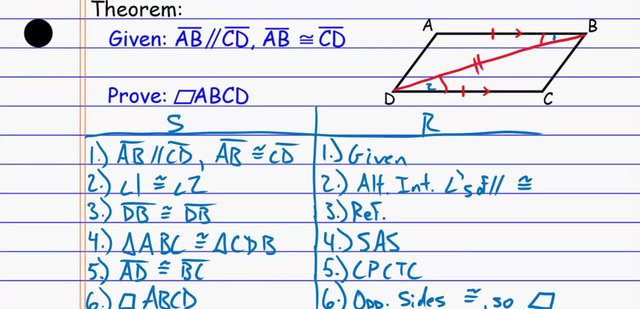 By proving this now I have one more way that I can show that these are parallelograms, and this way doesn't require both pairs of opposite sides. It only requires one pair, but as long as I know that that one pair are both congruent. 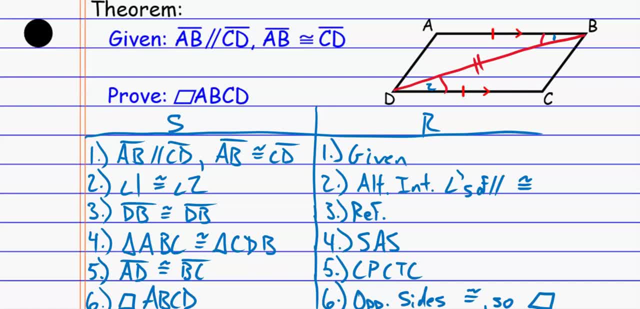 and parallel. I can say that it's a parallelogram. Okay, And really, when you think about it, we need four things in each of these. Okay, I need two pairs of stuff. all right, whether it's both pairs of opposite sides congruent. 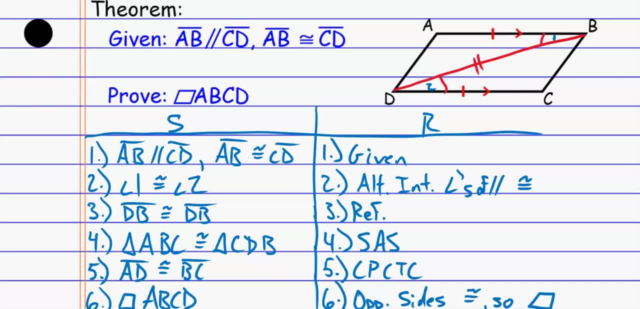 or both pairs of opposite angles congruent or just one pair. but I need two different things. I need that pair to be congruent- that's two things- and that same pair to be parallel- Okay, So if a quadrilateral has one pair of opposite sides that are both parallel and congruent, 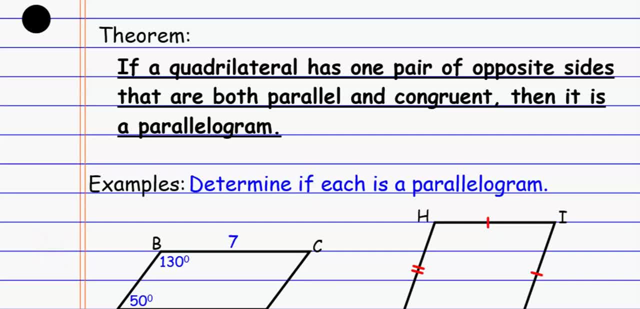 then we can say that this thing is a parallelogram. Okay, So we have all of those properties that we can use in reverse, all right, to show that it's a parallelogram. And then we have this special one where I just look at one pair of opposite sides and 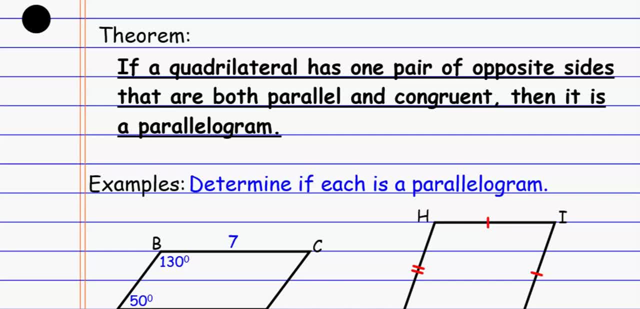 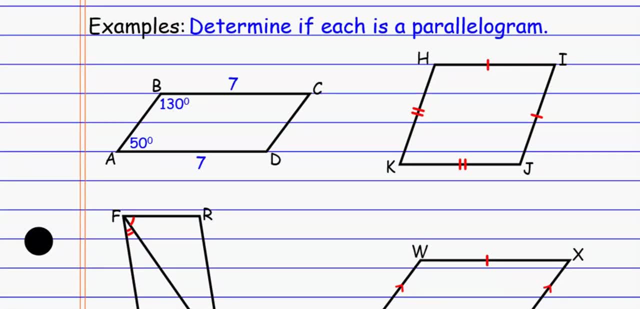 if they're both congruent and parallel, then I can say that this thing is a parallelogram. Okay, And now? if I look at these, let's determine if each of these is a parallelogram. And I might not be able to determine if it's a parallelogram. 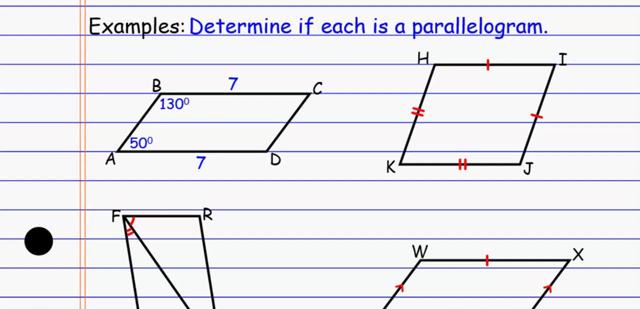 And so, as I look at this, let's look at the information I have. So, this one, I'm given these two angles, and given that these two angles are supplementary, the thing is, though, I can't use that rule that says: you know, oh okay, I'm going to. 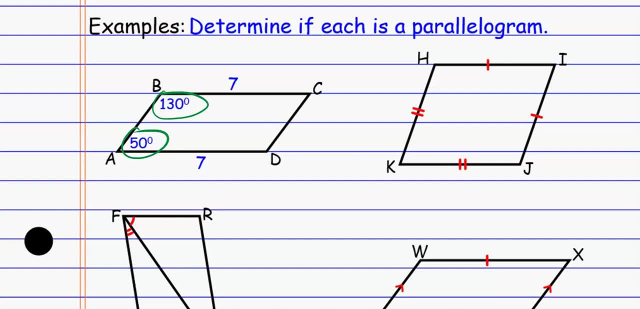 do this because you know if both pairs, if two pairs of consecutive angles are supplementary, because I would need this pair to be supplementary as well. Okay, So because I only have one of these sets, the only thing that that tells me is that 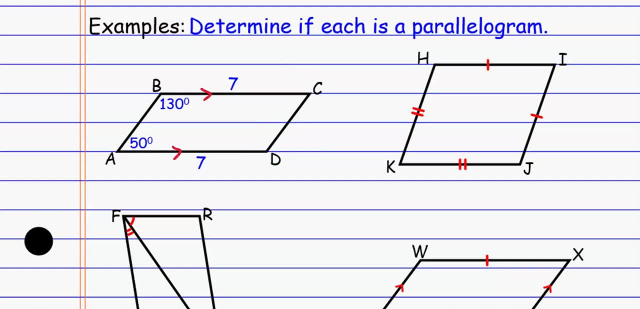 the opposite sides is that this guy is parallel to this guy. Okay, And I can say that those are parallel because they're same side interior angles. But now I have one pair of sides- BC and AD- that are both parallel and congruent because 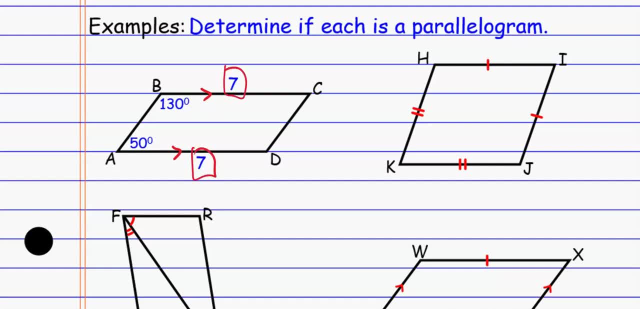 of the sevens. So I can still say that these are, that this is a parallelogram, but maybe not for the reason that you originally thought. Okay, So I can say that this is a parallelogram because of that special theorem that we just 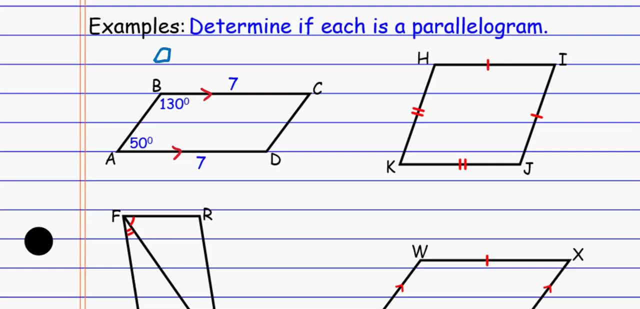 that we've just proven, Okay. So the yes, this is parallelogram ABCD And it's because of. so make sure you understand the justification. it's because of I have one pair of opposite sides that are parallel and congruent. 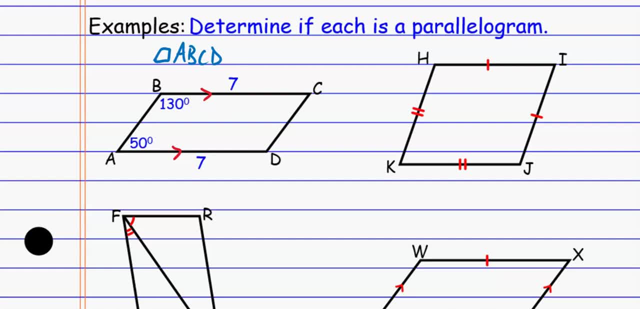 Okay, If I look at the next one, I noticed that I have these sides congruent and then, separately, I have these sides congruent, but those are not opposite sides. These are not opposites. These are not opposites. Okay, So there's not really much I can do here. 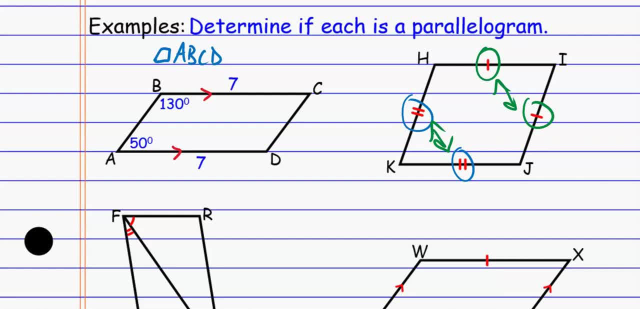 I don't know anything about the angles and I don't have the opposite sides congruent, So I cannot prove that this is a parallelogram. Okay, So I'm just going to write: no, Okay, Not enough information can't be done. 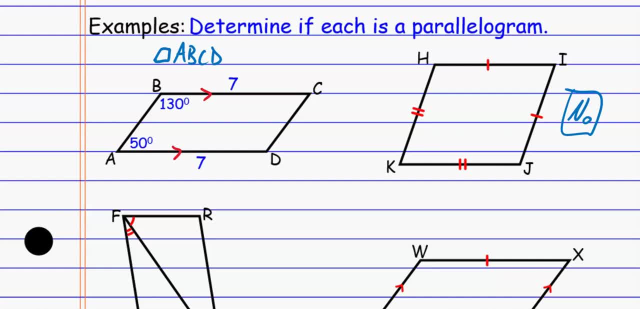 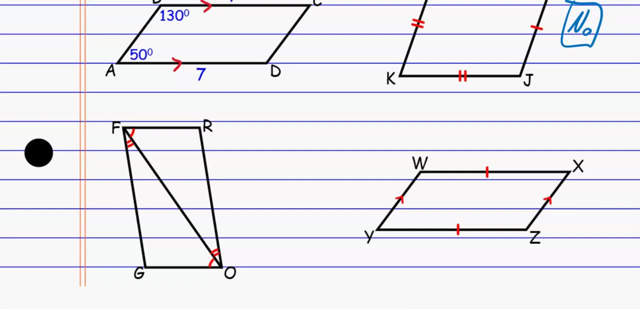 All right, Not enough information here. If all of those sides were congruent then I could say it's a parallelogram If I look at this guy, same kind of thing as I look at this when I look at the angles. 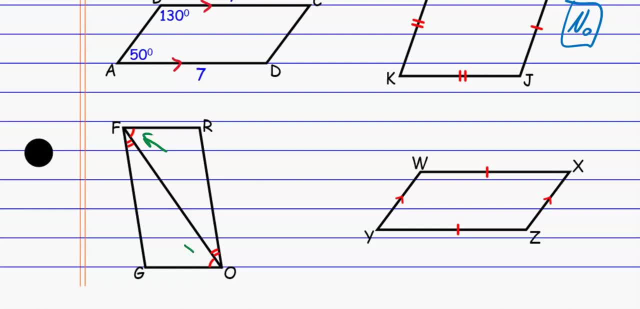 that I have here. So, looking at these two angles, okay, being congruent, if those two angles congruent, those are alternate interior angles for these two sides, which means by those being congruent. I know that these sides are parallel. 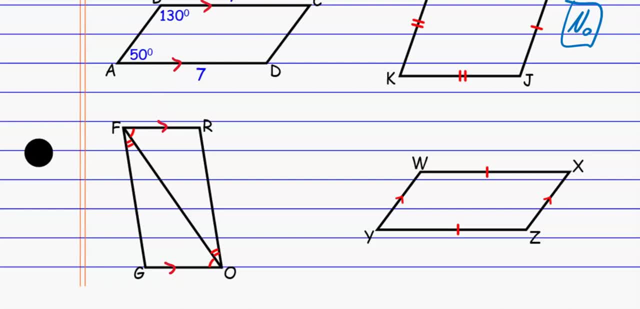 Okay. And then if I look at the other pair right here, these guys being congruent, well, those are alternate interior angles of these two sides. So by saying that those are congruent, I could say that these two sides are parallel. 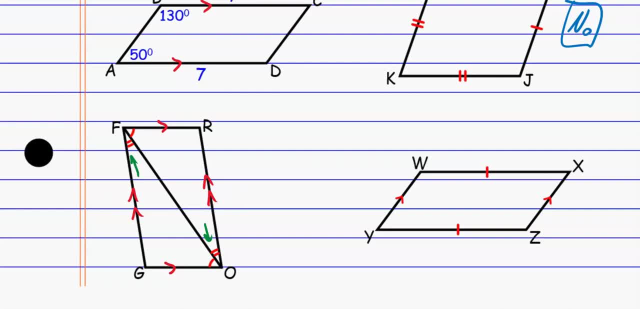 Okay, And notice, I don't have opposite angles of the parallelogram congruent. What I have are angles that give me the sides being parallel, And so as I look at this one, I can say that this is a parallelogram. 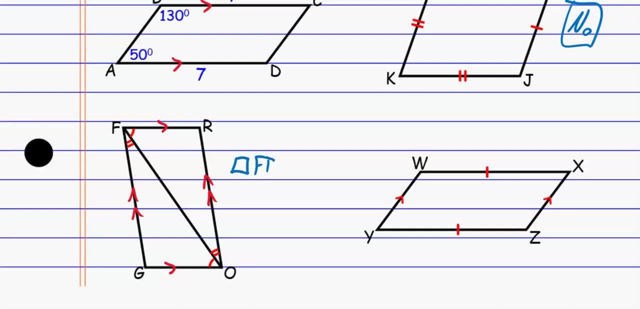 Okay, But my justification is the definition of parallelograms, because I have opposite sides parallel. Okay, If I look at this guy, I have one pair of opposite sides that are congruent and a separate pair that are parallel, And so students will tend to jump on this and say, oh, it's a parallelogram, because 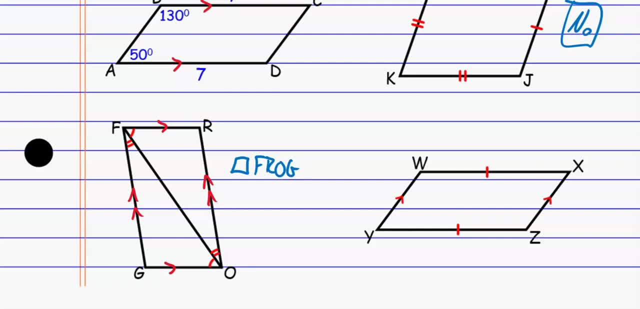 I have a pair that's opposite, a pair that's congruent and parallel, but it's gotta be the same pair, That special one. Okay, It's the same pair of opposite sides, both parallel and congruent, and these are different. 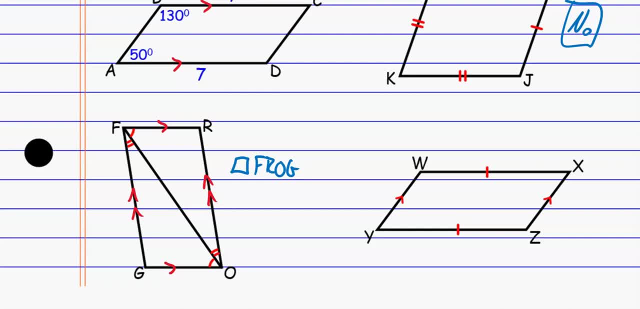 sides, Okay, And so maybe there's still a justification here. So maybe we start drawing some of this stuff and we start talking about, like these angles being congruent, But when it's all said and done, you know we don't have enough information here. 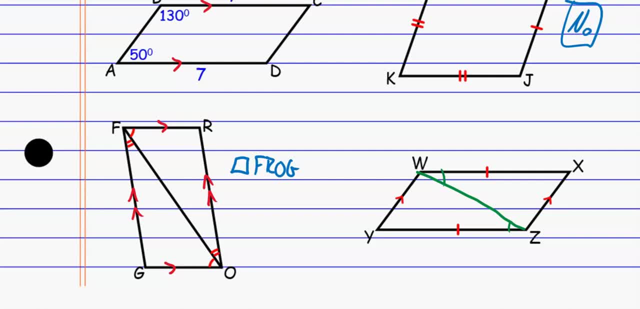 Okay, And so as we look at this thing, I've got those angles. I even have something like this side here, So maybe I could- I could go through a proof of justification Saying: hey, you know, I've got two congruent triangles here by side, angle side. 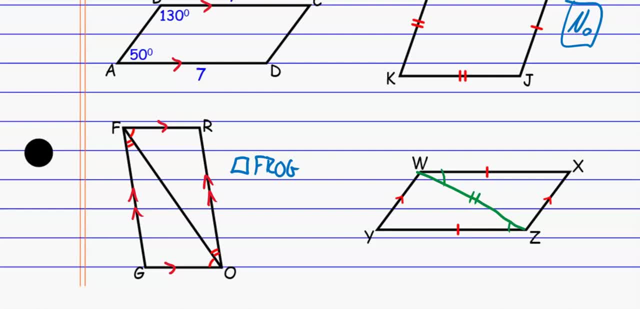 Okay, But really I don't have any of these properties, So I could maybe prove this to be a parallelogram through a proof of some sort, but I don't have it right away. Okay, And so this one I'm going to say: not enough information for now, so I'm just going to 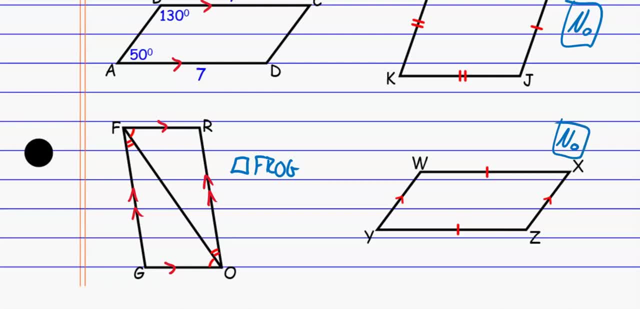 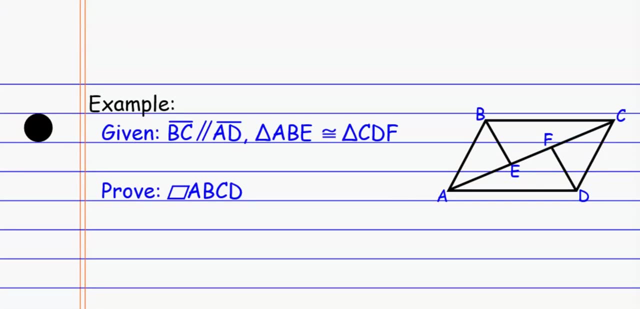 say no, Okay. Okay, This is one of the things that I have. Okay, Maybe I could go through a proof to come up with it, but I can't justify it using the things that we've discussed so far. Okay, If I look at this guy, we're going to construct a proof this time. 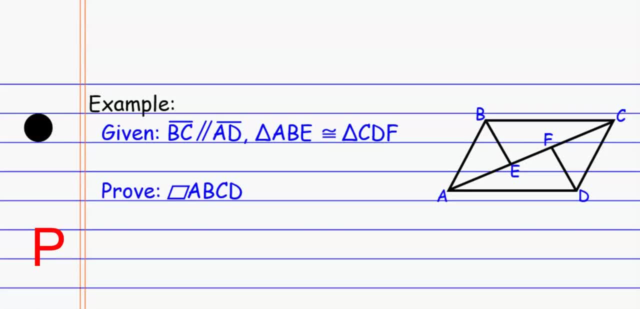 And I've got BC is parallel to AD- Let me label that on my picture- And I've got triangle ABE is congruent to triangle DEF. So it's this little triangle here and this little triangle here. They are congruent. And now from here I want to prove that this whole thing, that the bigger picture, the 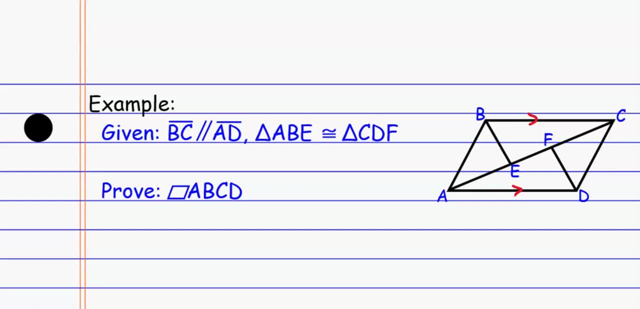 ABCD is a parallelogram, And so start thinking about what we know. We already have a pair of parallel sides, So maybe I'm thinking could I show that that same pair of sides, BC and AD, are congruent? because that would give it to me. 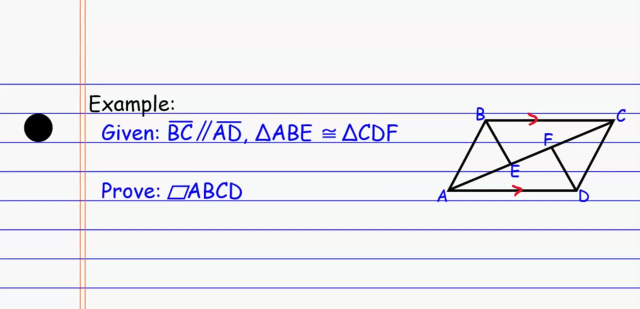 Okay, Or maybe I could go the route of the definition and try to prove that AB is parallel to DC. Okay, Or maybe I could, Okay, Or maybe I could prove that BC is congruent to AD, Or maybe that AB is congruent to CD, that kind of thing. 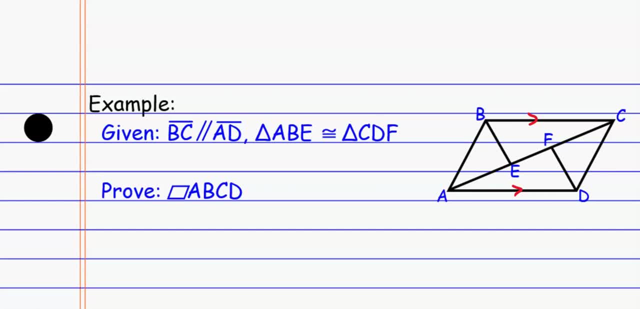 So we're kind of looking for our options here, And really the two that make the most sense are trying to prove that BC is congruent to AD or trying to show that AB is parallel to DC. Okay, So go in the route of that special theorem or go in the route of the definition. 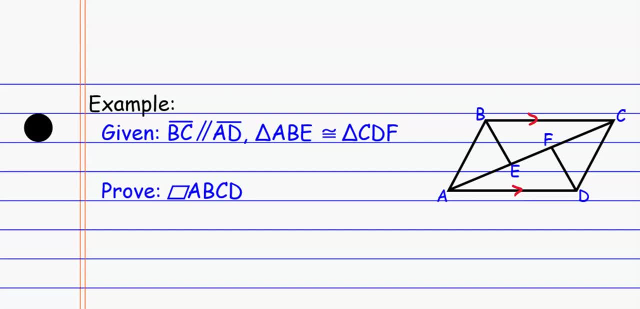 And so let's think about what we know. as I start to think about knowing that the two triangles are congruent, Well, right away, I would know that, like these guys are congruent because of CPCTC or these guys or these guys, And maybe you're looking at that thinking, well, I don't know if that really helps me. 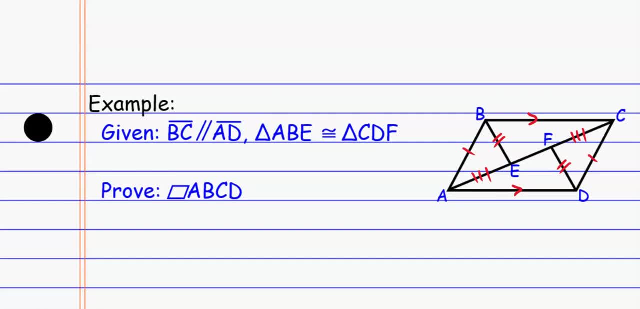 or not, But maybe you would look at something like this and say, hey, this angle, angle one and angle two would be congruent because of CPCTC, And so as you look at that, hopefully you recognize that those are alternate interior. 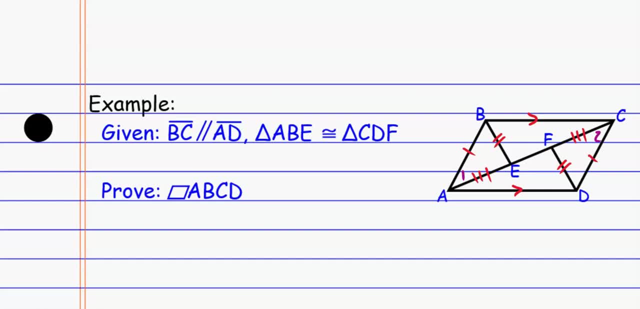 angles for lines AB and CD, which would make them parallel. Okay, And so let me erase all the stuff that's probably not going to help me If I think about just that information that would give me opposite sides parallel, which would give me this thing through the definition. 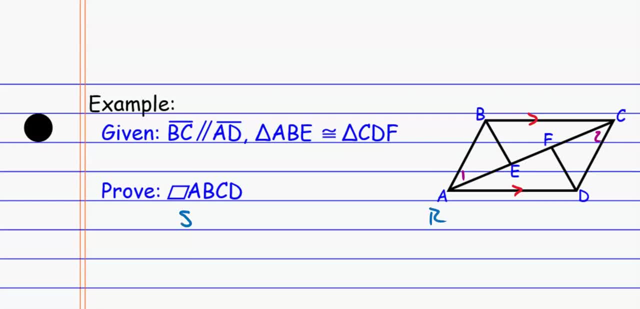 And so let's kind of construct the proof off of that. And so, again, I'm just kind of thinking about what I know to try to figure out. all right, do I have a path to this thing? And then, constructing the proof, we're just going to write out that path. 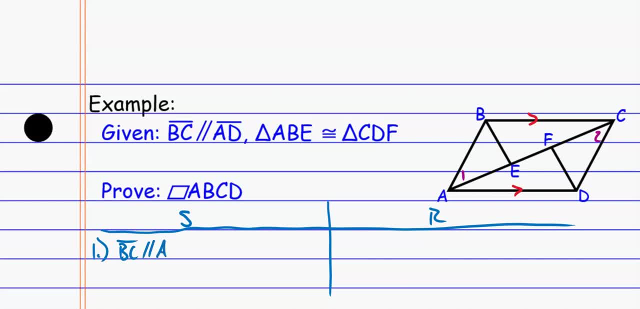 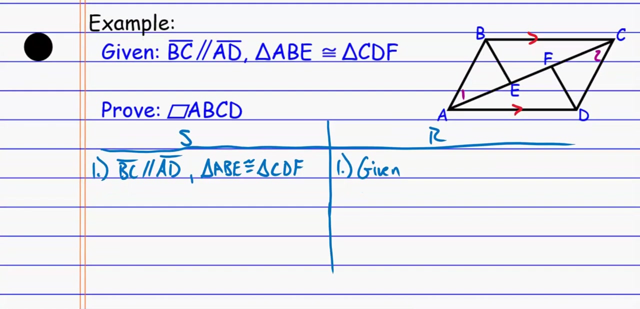 Okay, Let's see BC is parallel to AD. Okay, And triangle AB is congruent to triangle CDF, And all of that is given. so I'm just going to say given here, Okay, And then from here let's talk about what we discussed. 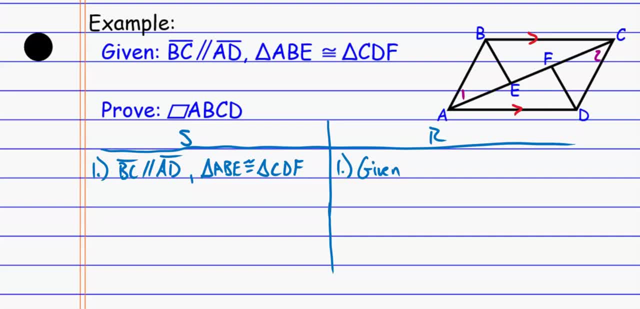 We said: hey, you know what? let's talk about the fact that angle one is congruent to angle two, And yeah, I labeled them that way. But angle one is congruent to angle two. Okay, And that's because of CPCTC.